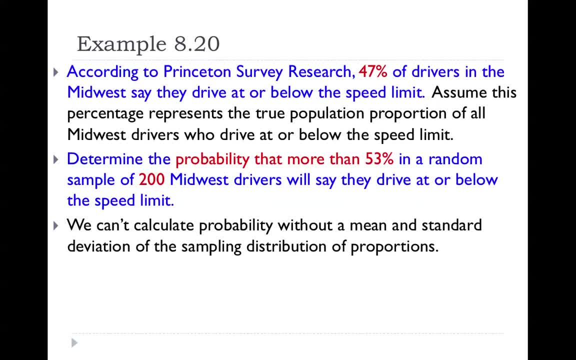 considered a sample proportion. So we can't calculate probability without a mean and standard deviation of the sample. We can't calculate the sampling distribution of proportions. We need to specify the center of the distribution. We need to know the mean and the standard deviation, or the mean and the standard error. 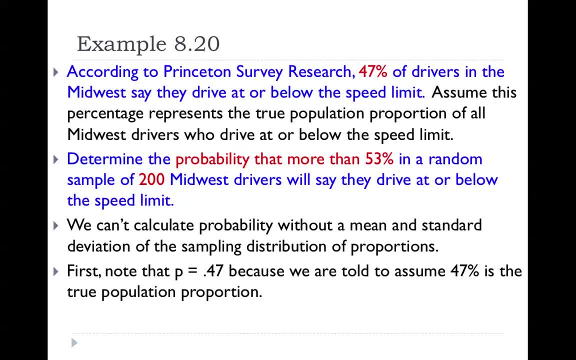 So since p is 0.47, we can calculate the mean of the sampling distribution just by knowing that mu sub p hat equals p. So mu sub p hat equals p, which is 0.47.. So our mean of the sampling distribution is 0.47. 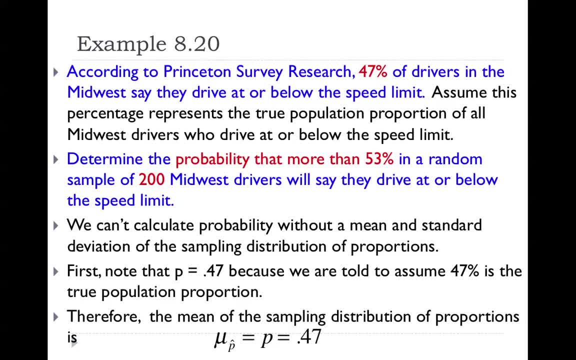 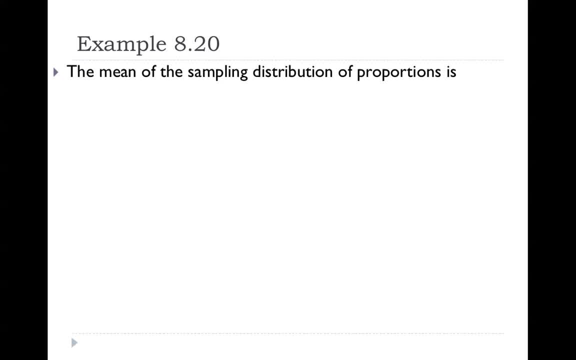 So our mean of the sampling distribution is 0.47.. So our mean of the sampling distribution is 0.47., Which is going to be the center of the bell curve. And now to calculate the standard error, we're going to use that formula again. 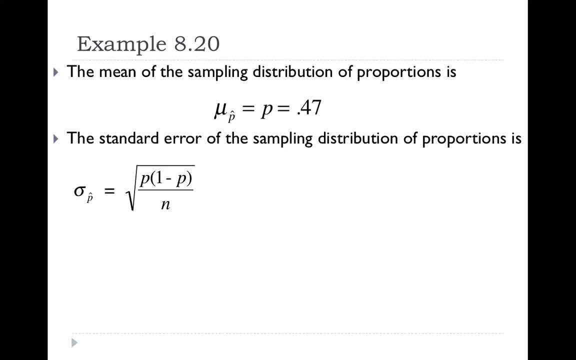 The square root of p times 1-p divided by n. Remember that p is 0.47.. So 1-p, we're going to take 1-0.47.. And n is 200.. we have a sample of 200 drivers. so let's go to the calculator. I'll do it together. 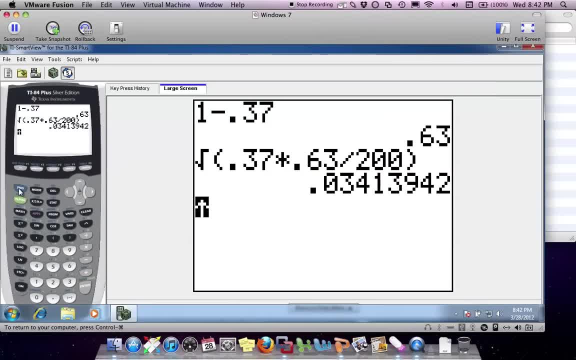 and we have the square root of. well, actually, before we do that, you may want to decide what the you may want to figure out what 1 minus 0.47 is okay, 0.53. so you've got the square root of 0.47 times 1 minus 0.47, which is 0.53. 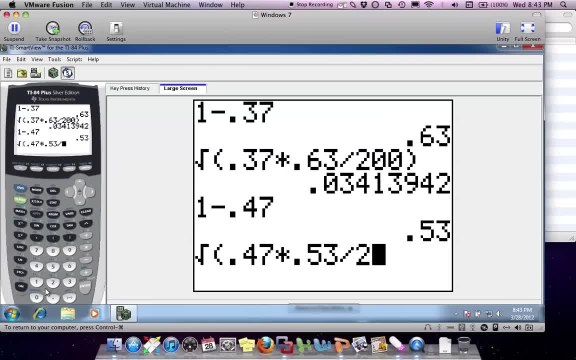 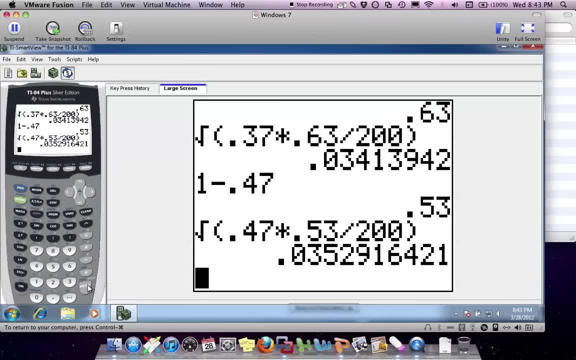 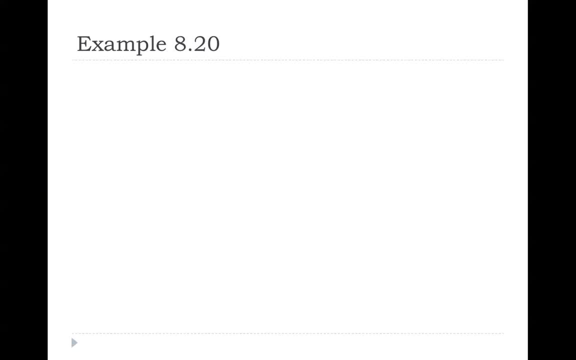 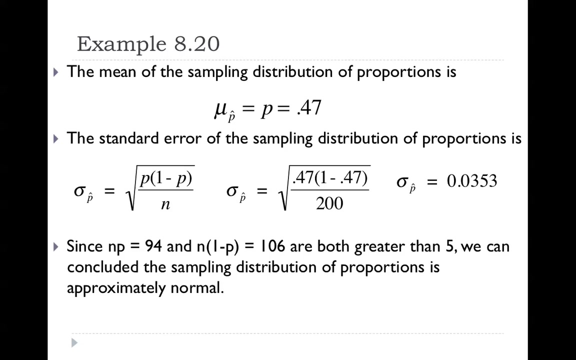 divided by the size of the sample. close the parentheses and you have 0.0353. okay, 0.0353. this is the standard error of the sampling. distribution of proportions. if you multiply NP, you'll get 94. this is if you take 0.47 and you. 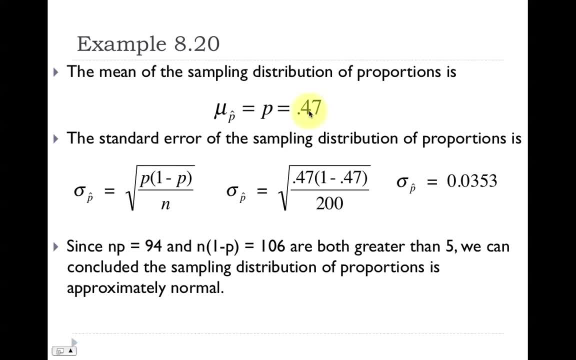 multiply it by 200- the size of your sample: 0.47 times 200, you'll get 94. if If you multiply 0.53, that's 1 minus p times 200, you'll get 106. Both of those are greater than 5.. 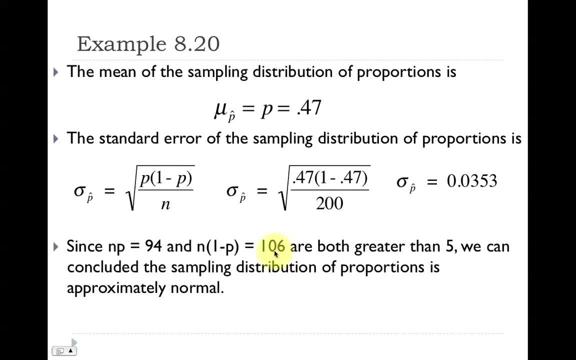 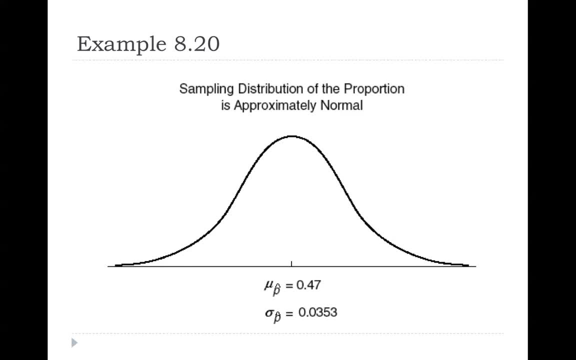 Therefore, you can use the bell curve, You can use the normal distribution to answer this question. Okay, so let's look at our bell curve. In the center of our bell curve, we have the mean of the sampling distribution of proportions and the standard error of the sampling distribution of proportions. 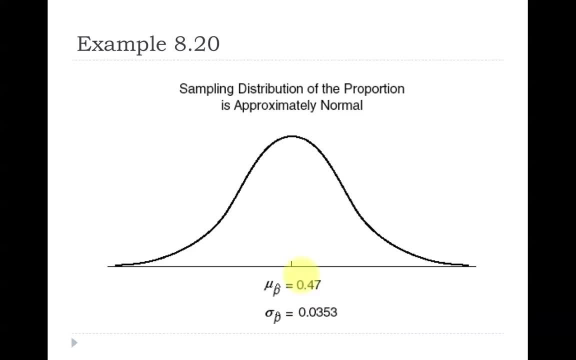 So we have 0.47 and 0.0353.. The values that make up the horizontal axis are sample proportions. Okay, so a sample proportion that's greater than 0.47 is going to fall to the right of 0.47,. 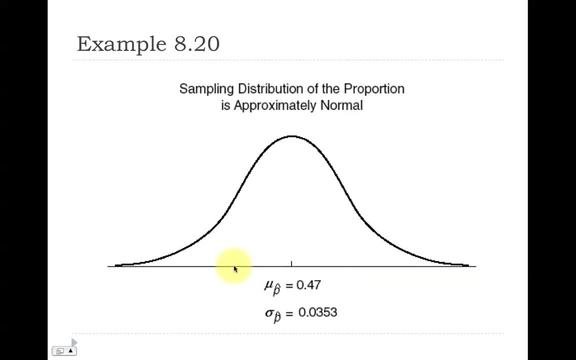 and a sample proportion that is less than 0.47 is going to fall to the left of center. The question is asking us to find the probability that more than 53% in a random sample of 200 will say they drive at or below the speed limit, which implies that 53% is p-hat. 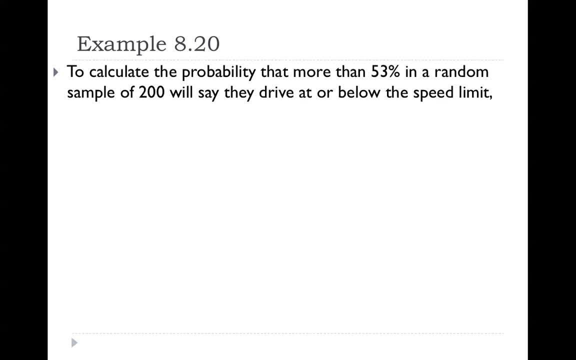 p-hat. the sample proportion is 0.53.. Okay, what we're doing is going to calculate the area underneath the normal curve to the right of 0.53.. This is the area that is greater than 0.53. 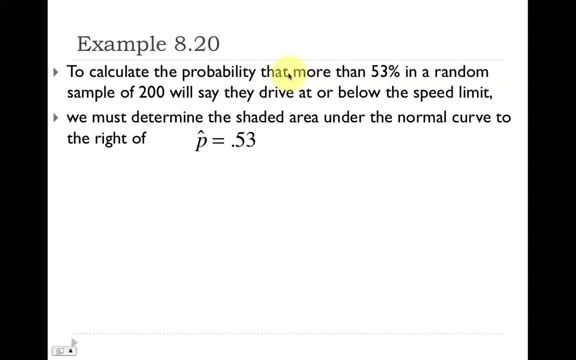 Why are we doing to the right? Because we're trying to find the probability that more than 53% More than means area to the right. So here's our bell curve. now, In the center, we keep our mean of the sampling distribution of the proportion. 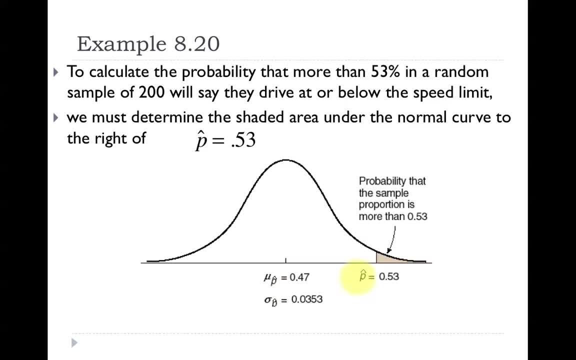 and standard error of the sampling distribution of proportions p-hat, p-hat, p-hat, p-hat, p-hat, p-hat, p-hat. The p-hat that we're concerned with is 0.53, and it is to the right of 0.47. 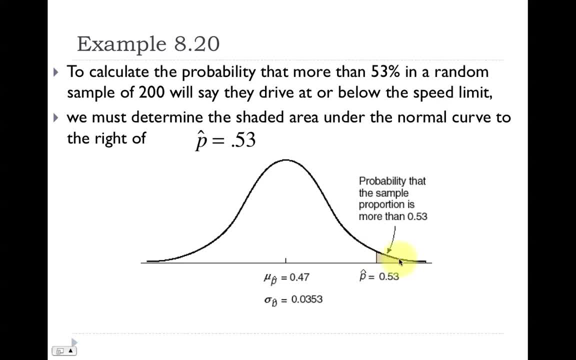 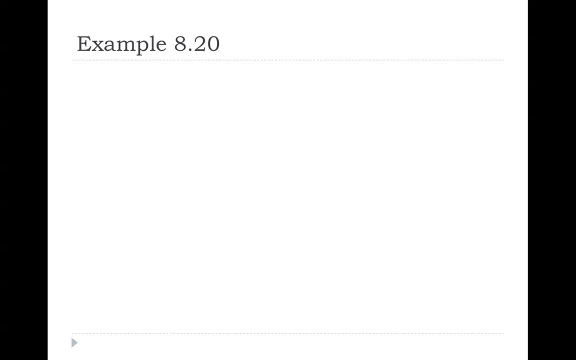 We shade area to the right of 0.53 because we're looking for more than 0.53.. Now into our calculator we're going to put in normal CDF again. We're going to use lower sample proportion comma, upper sample proportion. 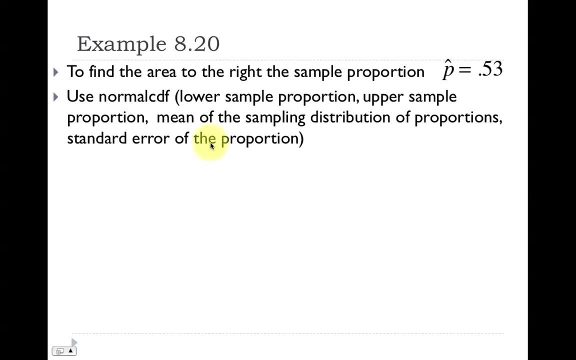 comma: the mean of the sampling distribution of proportions. comma- the standard error. Okay, so these are our values. We're going from a p-hat of 0.53 up to positive infinity. The mean of the sampling distribution of proportions is 0.47,. 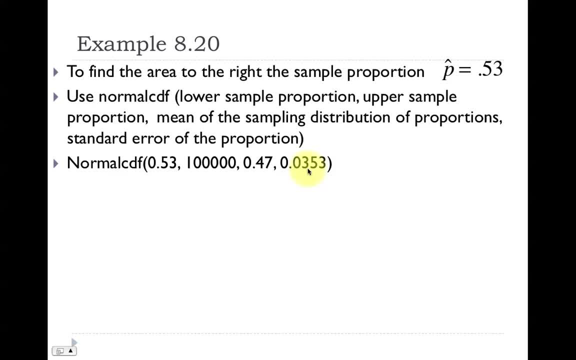 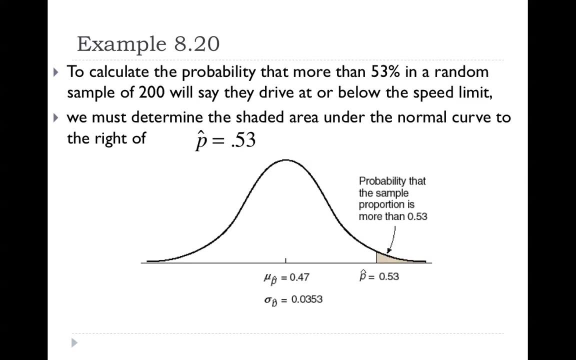 and the standard error that we calculated is 0.0353.. So you should get 0.0446 or 4.46%. Okay, so the four values again that go into the calculator: p-hat: 0.53, comma positive infinity, which is way up here: 100,000,. 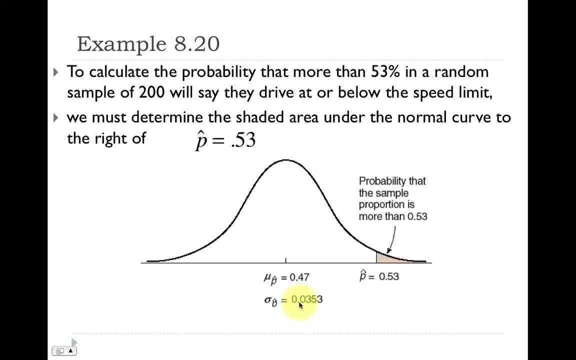 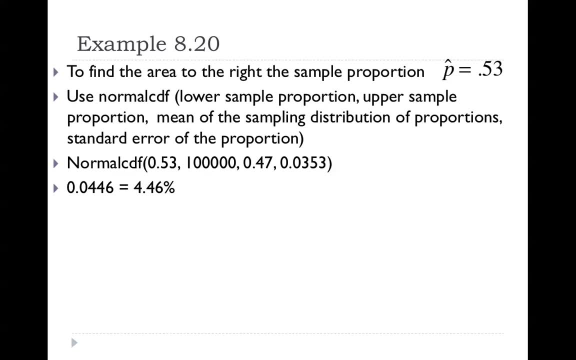 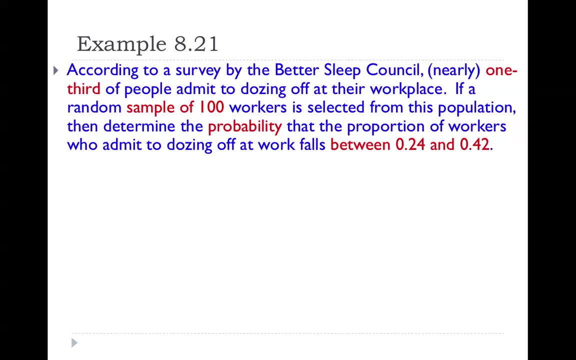 comma mean comma standard error and then hit enter and you'll get 0.0446 or 4.46%. Example 8.21.. According to a survey by the Better Sleep Council, nearly one-third of people admit to dozing off at their workplace. 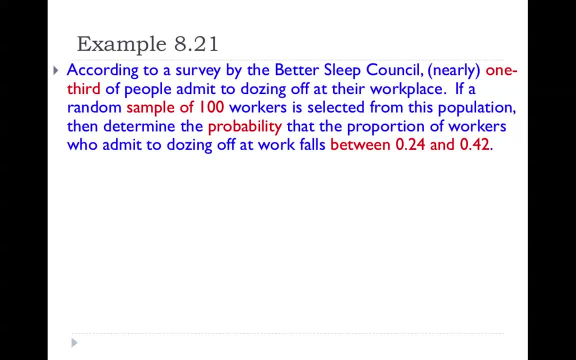 If a random sample of 100 workers is selected from this population, determine the probability that the proportion of workers who admit to dozing off at work falls between 0.24 and 0.42.. Okay, so a few things are being given. 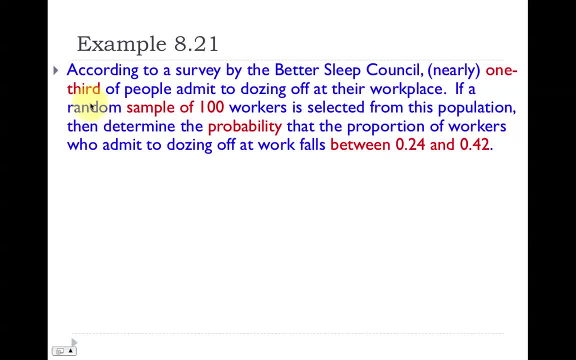 Given here in red. you see one-third of people admit to dozing off at the workplace. This is our population proportion. The size of our sample is 100, and we're trying to find the probability that the sample proportion is in between 0.24 and 0.42.. 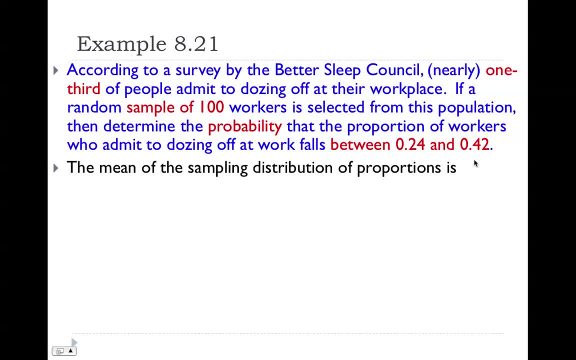 The same as the population proportion. The mean of the sampling distributions of proportions is always going to be the same as the population proportion. So we can take 1 divided by 3, which is approximately 0.33.. Our standard error is gonna be the square root of p times 1 minus p divided by N. 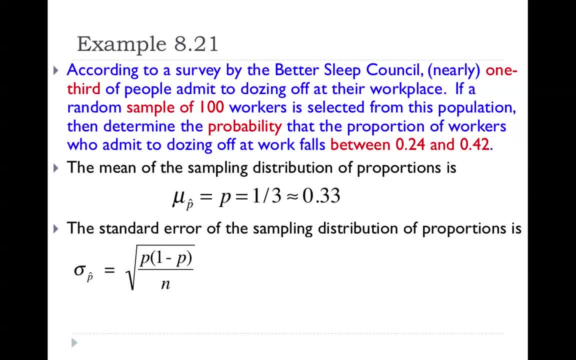 So we're going to take 0.33, times 1 minus 0.33, divided by n. so again on your calculator you may want to figure out what one minus 0.33 is. if you figure that out first, you've got 0.33 times 0.67 divided. 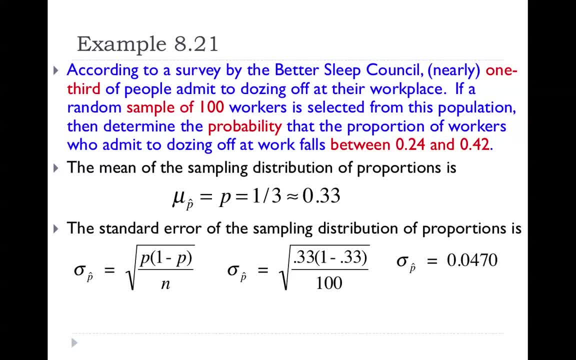 by 100, which is going to give you 0.0470. this is the standard error of the sampling distribution of proportions. so now you're going to label your bell curve. if you just do a double check, you can see that if you take NP, you get 33. 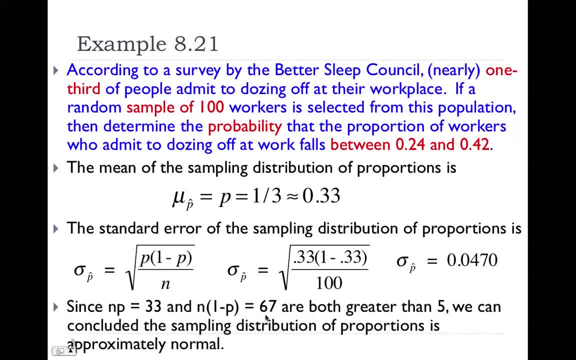 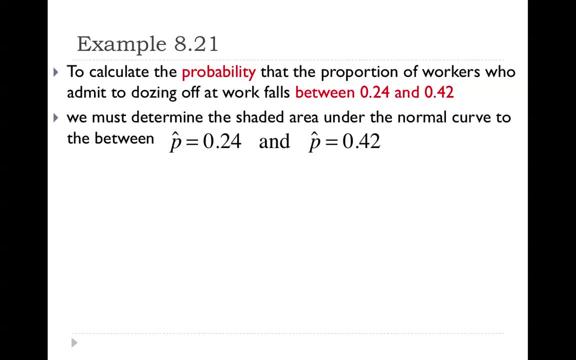 if you take n times 1 minus P, you'll get 67. both of those are greater than 5, so you definitely have a bell curve. the shape of this distribution is approximately normal. ok, so to find the probability, we're looking at area under the curve between a. 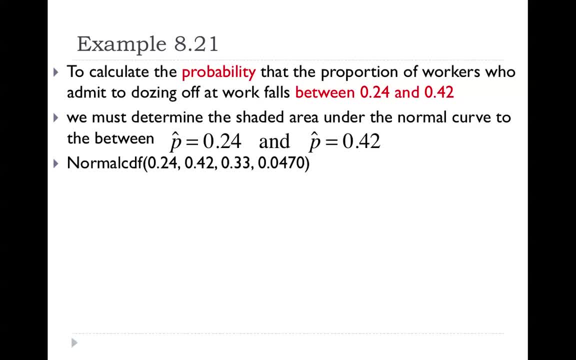 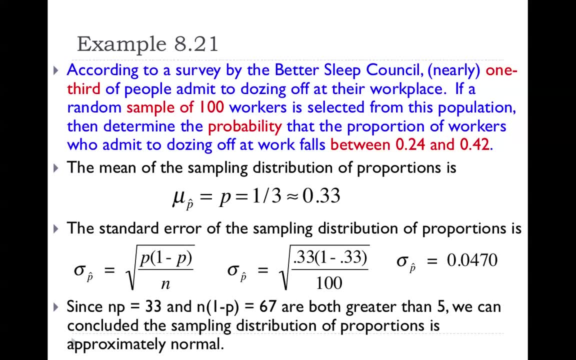 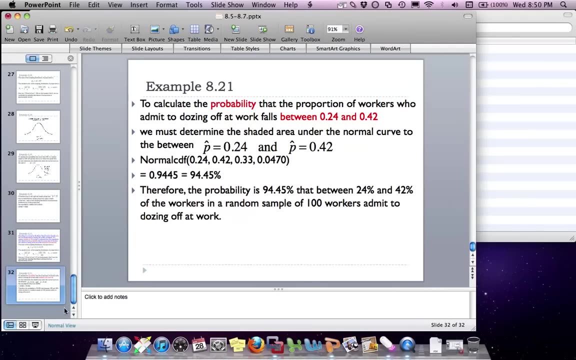 p-hat of 0.24 and p-hat of 0.42. so let's see, do we have a picture? ok, there's no picture in this problem, but what we're doing is identifying the lower p-hat. so 0.24 is lower than 0.42. 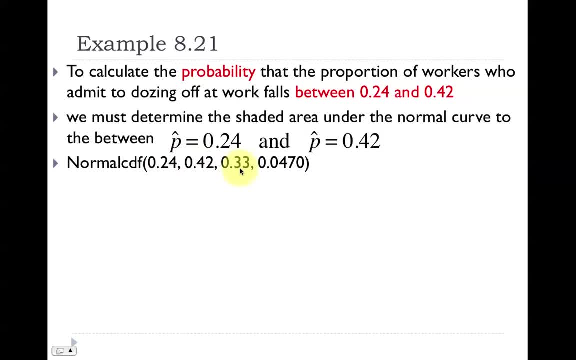 lower p-hat. comma 0.42 is the upper p-hat. the mean of the sampling distribution of the proportion is 0.33. the standard error 0.0470. hit enter and we should get 0.9445. 94.45 percent and that is the chapter on sampling.